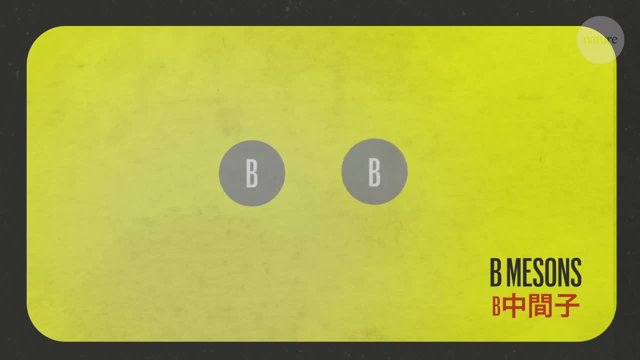 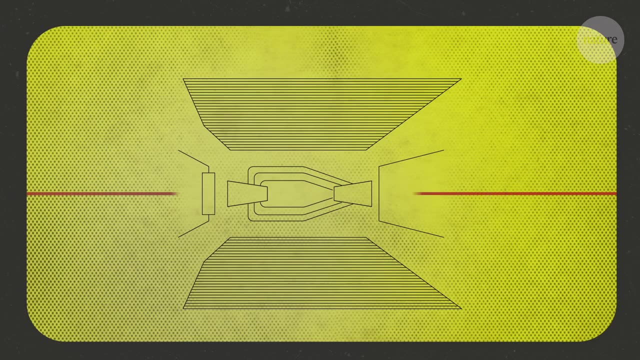 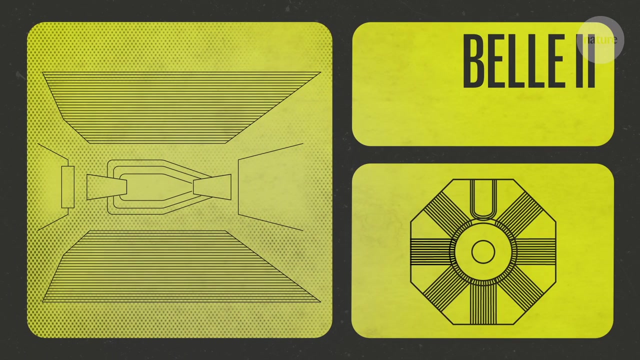 and annihilate each other, producing two B-masons. These unstable mesons immediately decay into lighter particles and fly away. By measuring these decays and the trajectories, researchers can look for places where the numbers don't add up, And that may be the key to explaining some of the big mysteries in the universe. 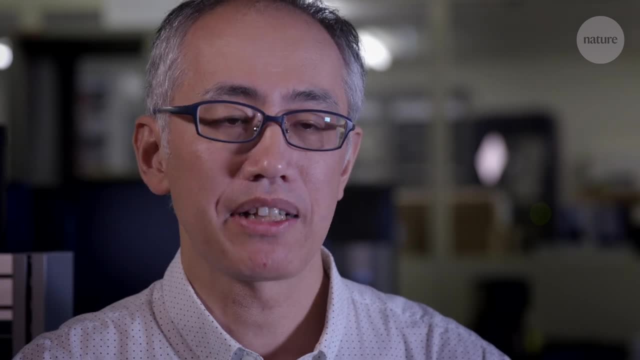 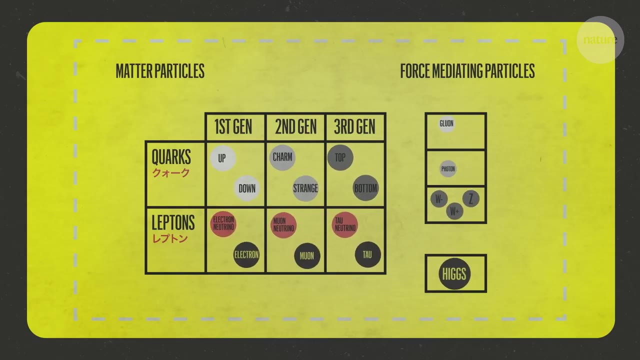 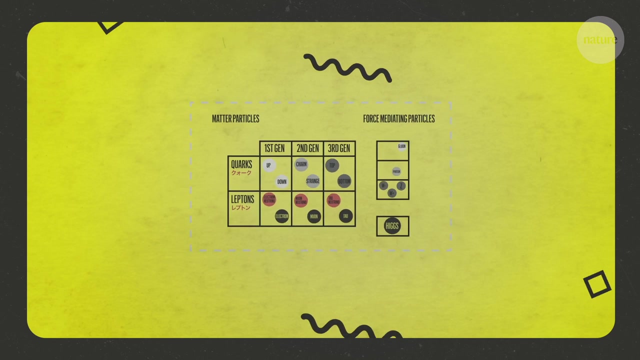 In particle physics. we have accumulated a lot of data and we have established the so-called standard model of particle physics, But this is still lacking a lot of things to answer the mystery of the universe. Physicists like Miki Hiko believe that there could be some new physics. 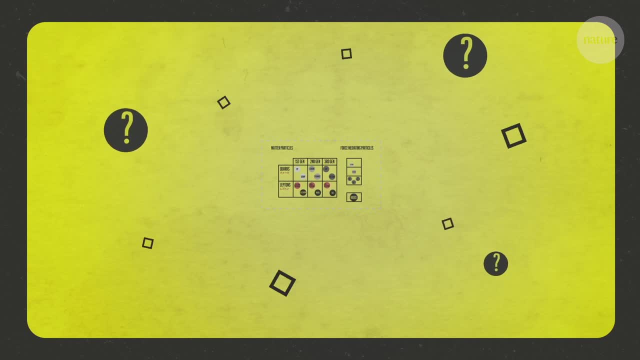 to discover which can explain some of these mysteries. One example is that no antimatter is observed in our universe And we don't know how this antimatter-matter imbalance was generated. at the very beginning, Something tipped the balance: some difference in behavior between particles and antiparticles. 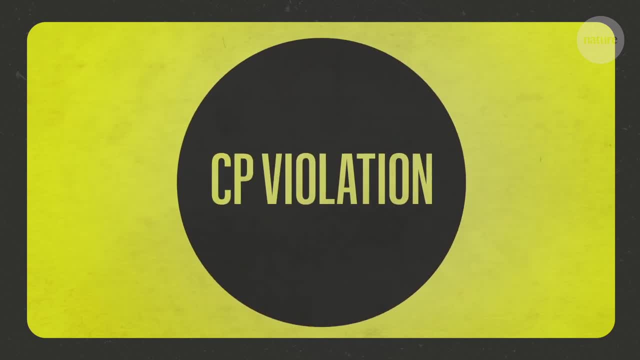 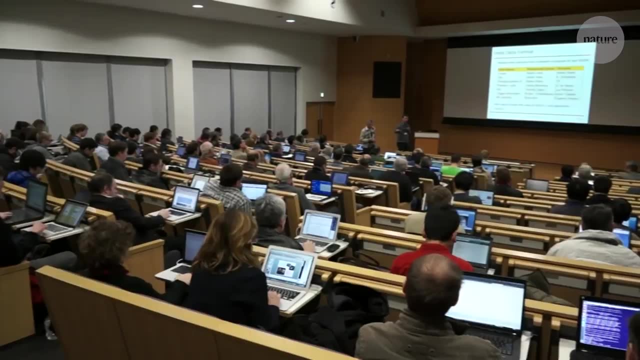 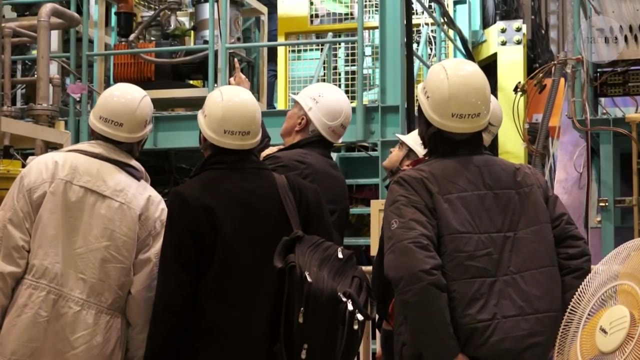 This difference is called CP violation, and it is one of the things BEL-2 is studying using B-masons. Back in 2001,, BEL, the predecessor to BEL-2, was among the facilities that first measured the CP violation in the decay of a B-mason. 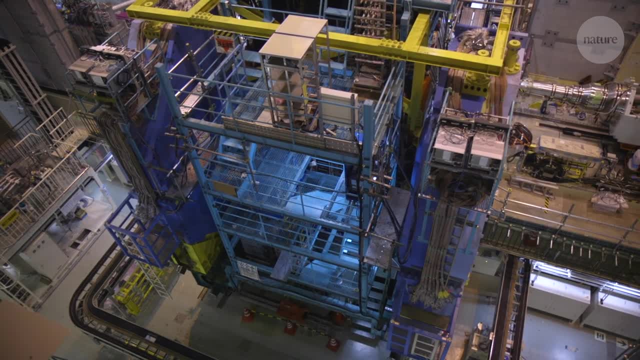 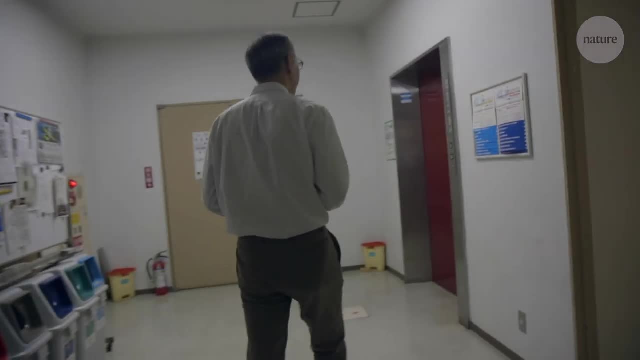 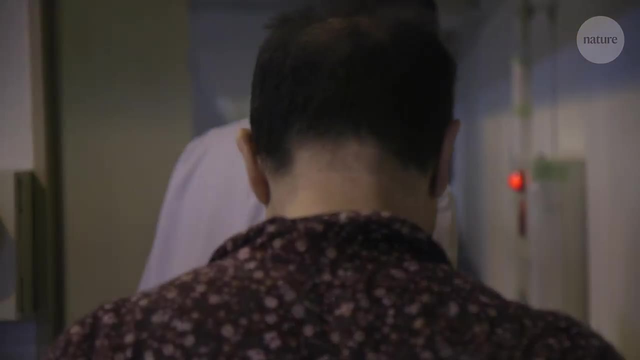 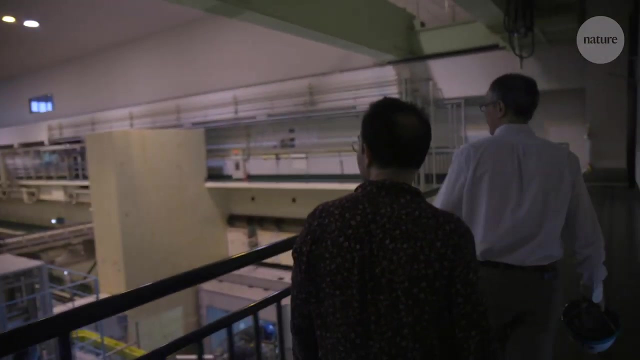 And BEL-2 is looking to confirm if those were hints of new physics or just statistical flukes. Miki Hiko took me on a tour of the detector to get a look at the engineering that makes this all possible- BEL-2. So now we are coming to the gallery area of the BEL-2 experimental hall. 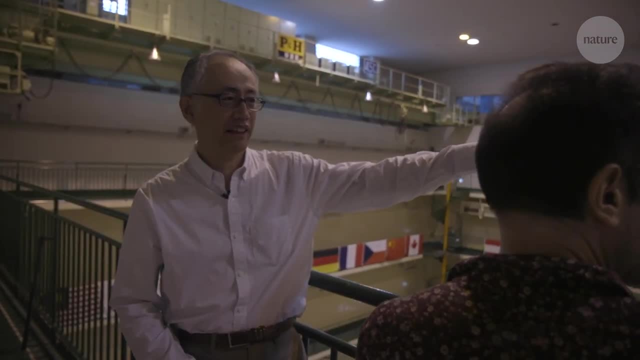 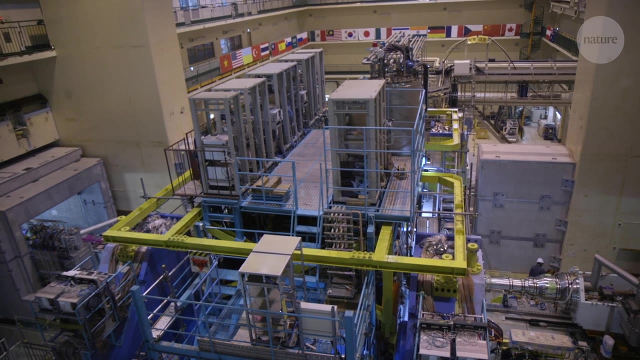 And usually we cannot go around the detector area, but because we are now in shutdown time, we are allowed to go there. The hall containing BEL-2 is vast and around the gallery are flags from every country that has collaborated on the experiment. 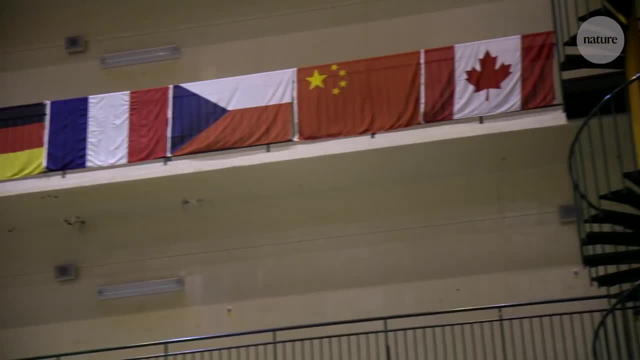 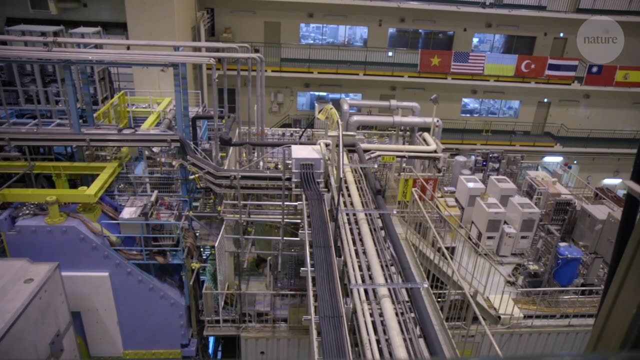 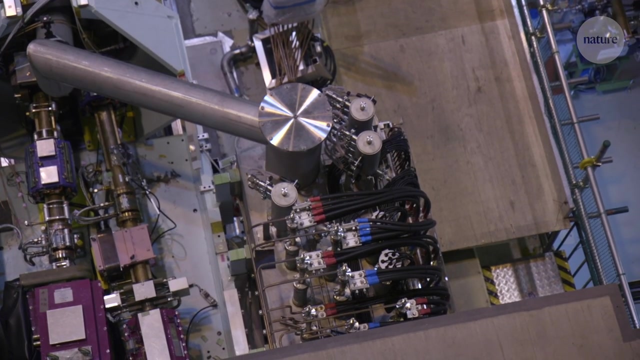 Over the years from Saudi Arabia to Vietnam. When I visited, the detector was still not fully operational. It had run some short tests, but it had been shut down again. So now we are on top of the beam line and you can actually see the two beam pipes. 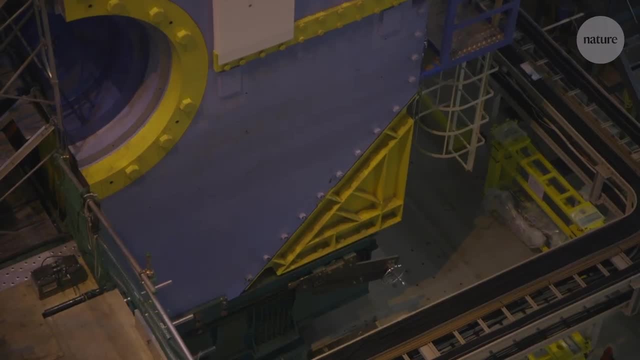 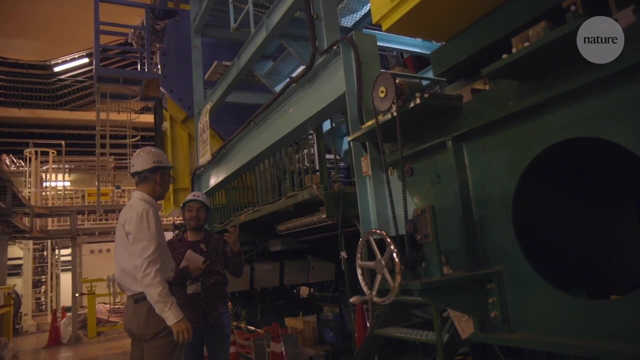 Huge metal yokes had been pulled apart and the detector had been almost totally deconstructed, which gave us a rare chance to look inside. Off to one side, in a clean space, researchers were testing the most advanced part of BEL-2,. 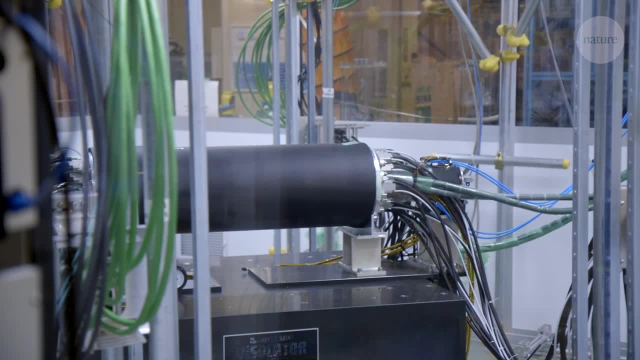 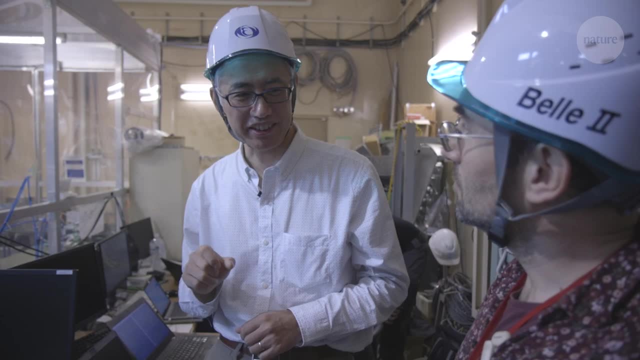 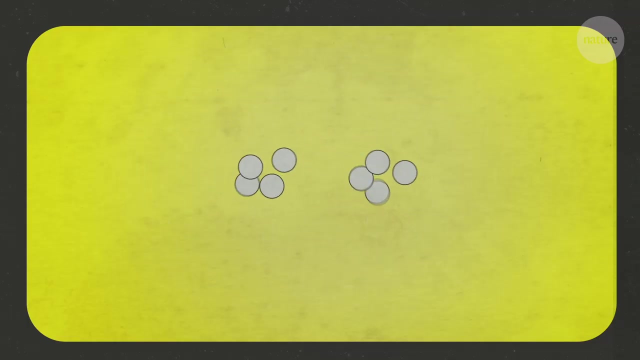 the silicon vertex detector. So this is the detector which can measure the origin of the particle at a resolution of less than 100 micrometers And this will go into the center of the detector. And it is by measuring these particles with incredible levels of detail. 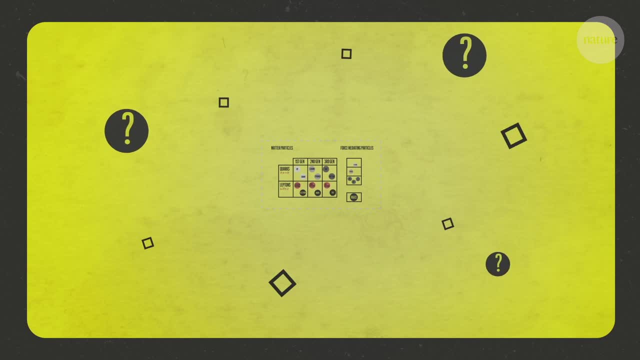 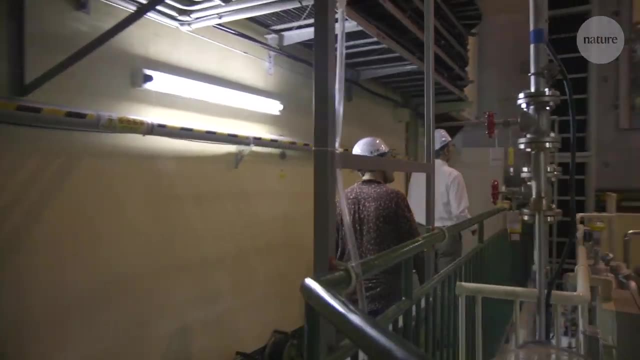 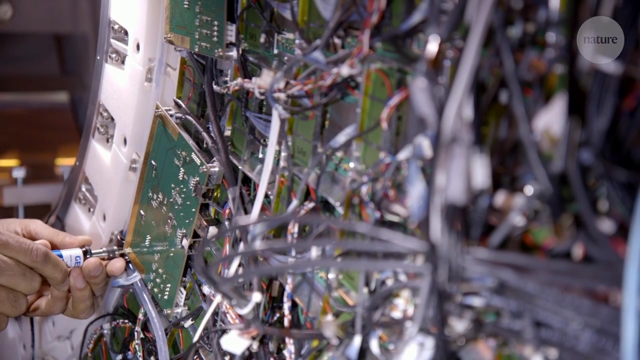 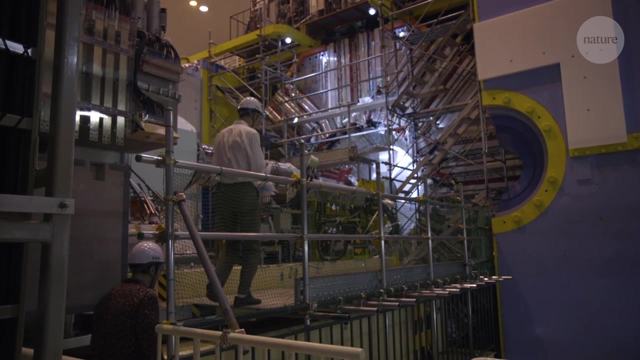 that Mikihiko hopes to discover new physics. As you approach the interaction point, you could see vast looms of wiring containing all the detection mechanisms which had been revealed. We were able to get closer than I ever imagined we would. In fact, it was a new experience for Mikihiko too. 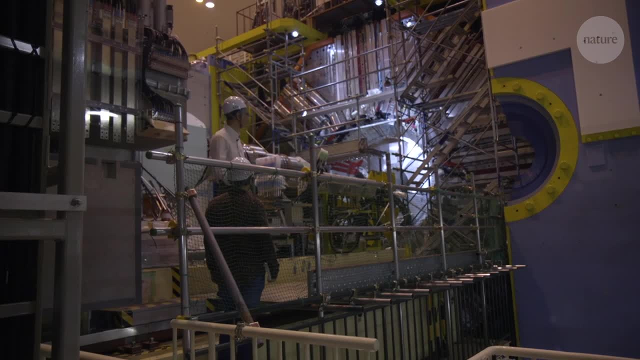 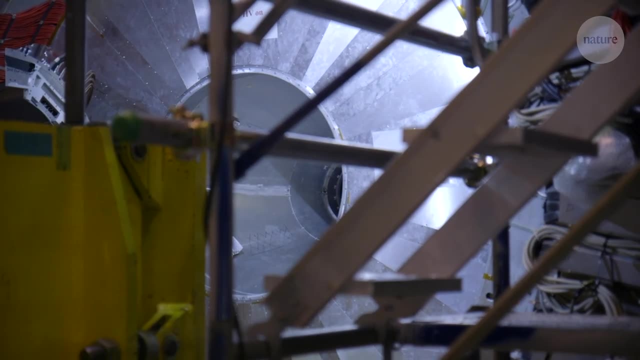 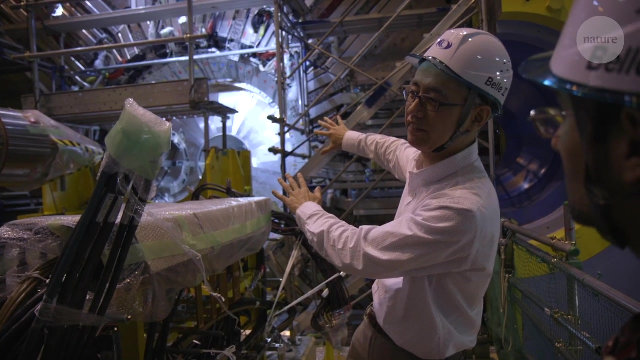 Actually, I'm not working in this area usually, so this is the first time for me to be here. We are in front of our BEL-2 detector and what we are seeing is that the end gap part is opened and end gap detectors are taken out. 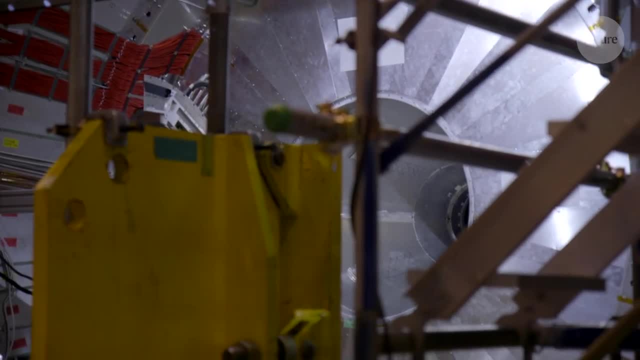 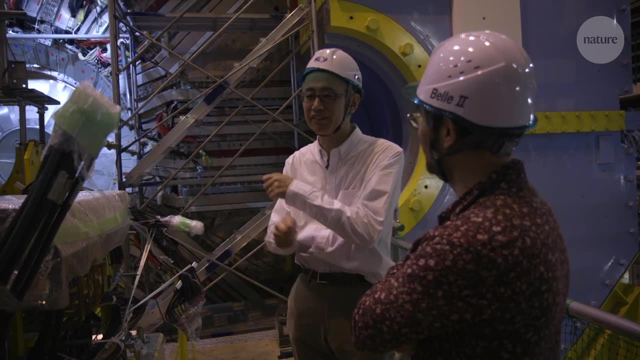 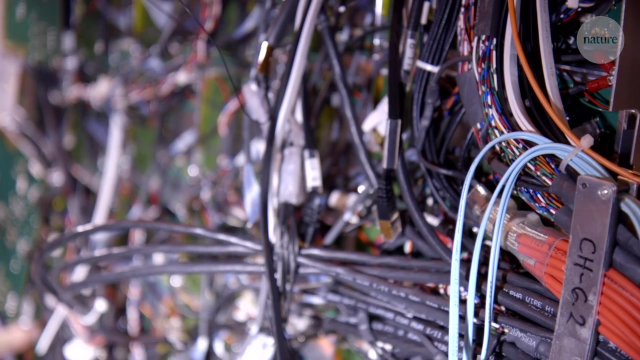 so that we can see the internal detectors, And inside there are like 40,000 wires. It's very often that people make the misconnection and they swap the cable in some places. If we are lucky, we can swap the cable on the other side too. 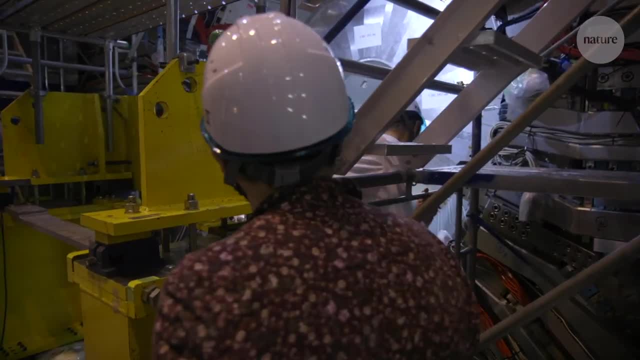 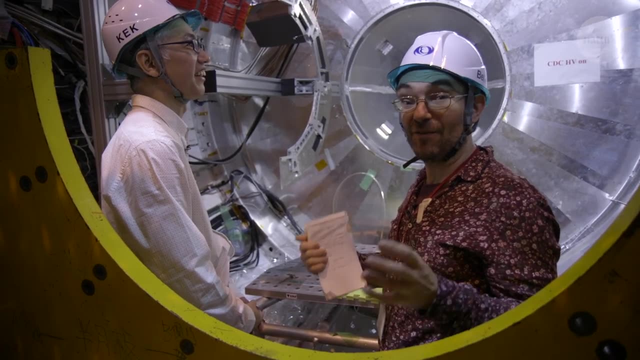 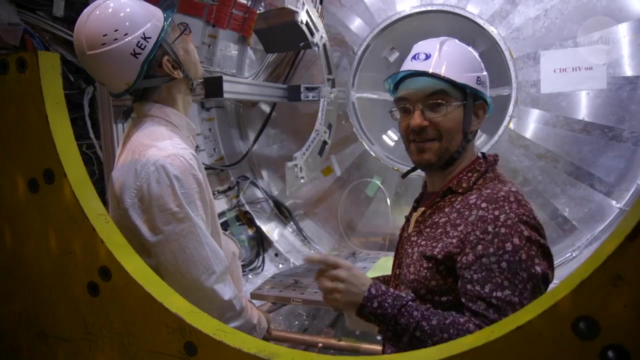 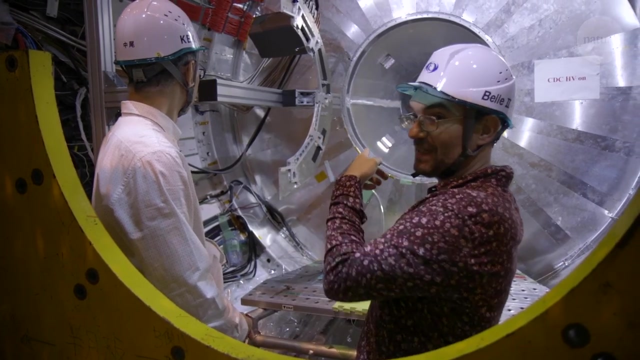 and everything is fine. So we're standing right in front of the heart of the BEL-2 detector. There will be the silicon vertex detector installed in the very middle, and then these two final focusing magnets will be inserted from the two sides, and that's where the electrons and the positrons will come. 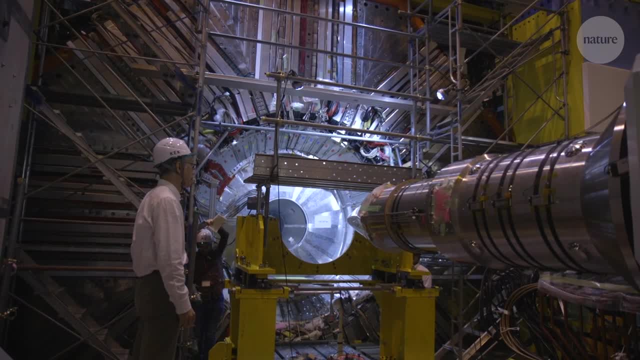 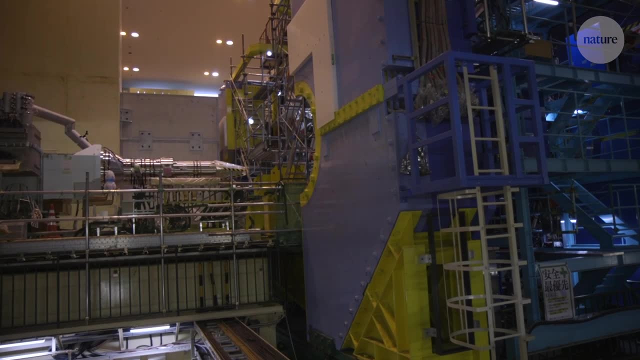 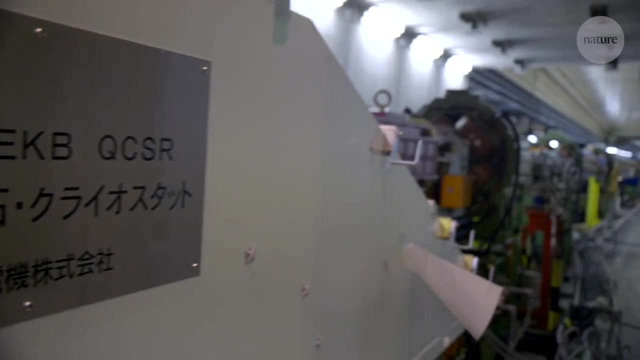 and meet at the interaction point. But before collisions can occur, first the researchers at KEK need to generate and accelerate the particles that come out of this tube, And to do that you need another vast piece of equipment, what particle physicists call the machine. 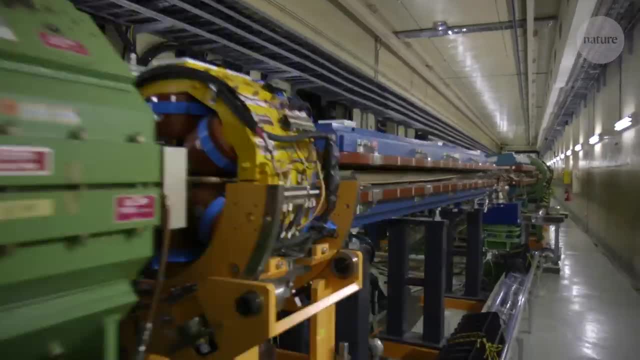 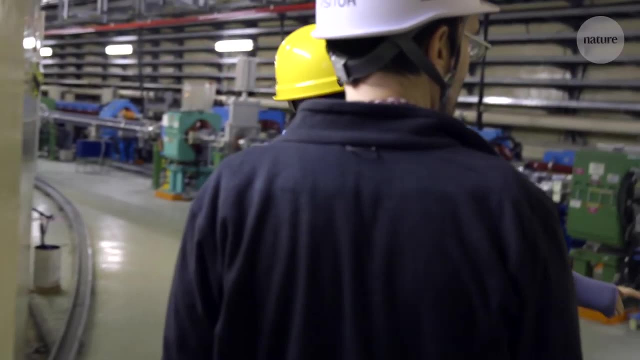 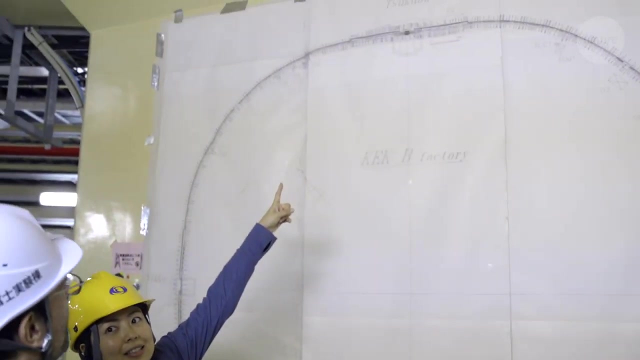 This is the accelerator, Super KEK-B. It took me on a tour of the tunnel that houses the beamlines, So we are here. We are here. Then the BEL-2 is there. So, yeah, this is a Super KEK-B accelerator. 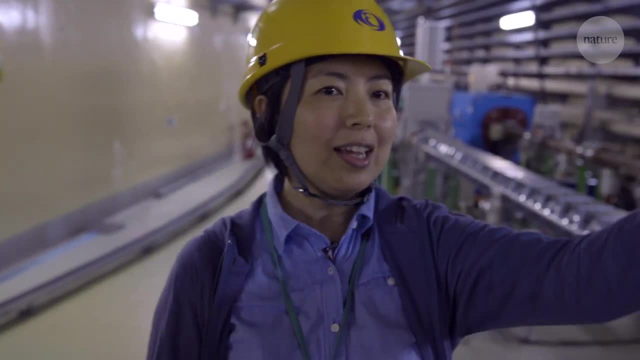 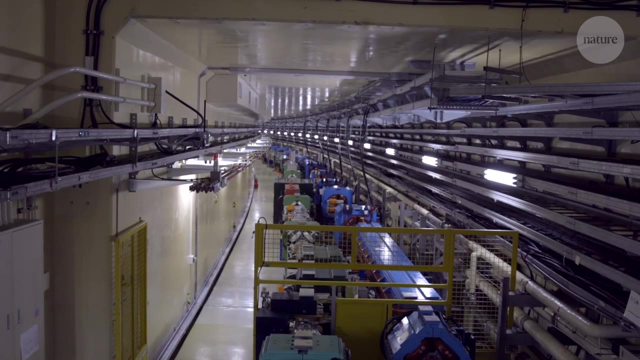 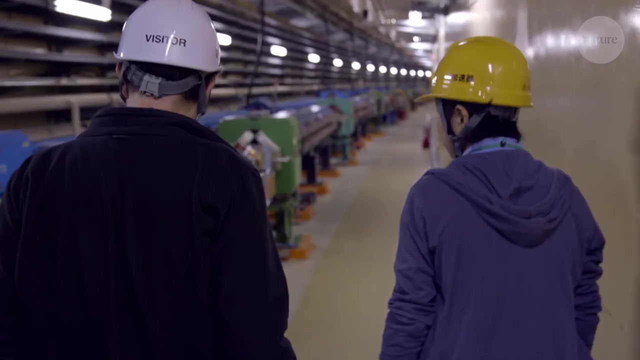 Then electrons come from there to there and positrons come from there to there. So in one tunnel we have two rings like this. Each ring carries either electrons or positrons, Matter or antimatter. They are accelerated to close to the speed of light. 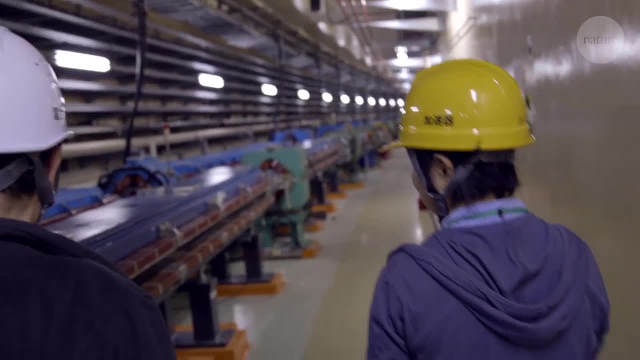 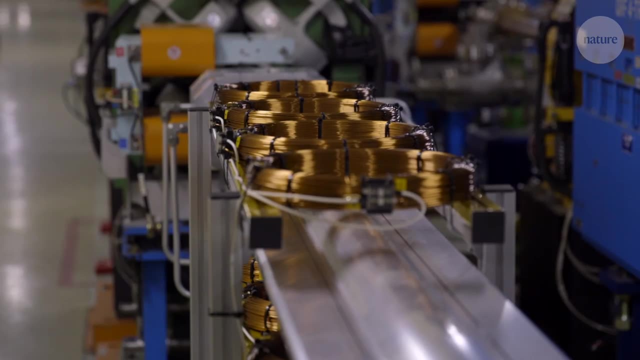 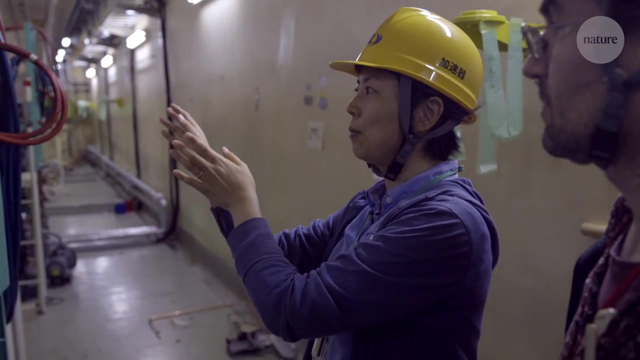 using powerful radio frequency waves and steered with a series of magnets placed all along the beamline. The list of equipment involved in creating, accelerating, shaping and maintaining the beam is mind-boggling. Injection beam- four injection beam- So large cavity- dipole. 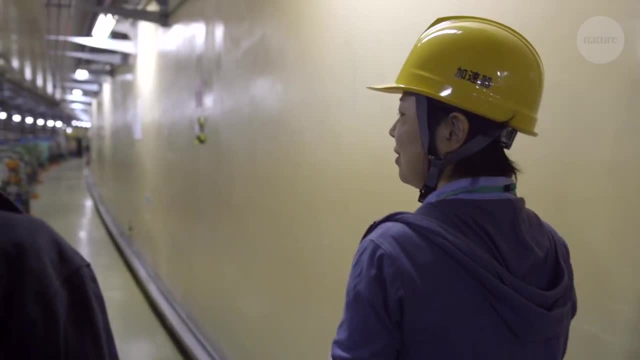 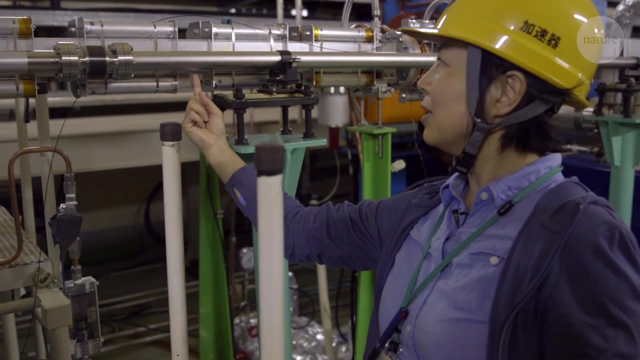 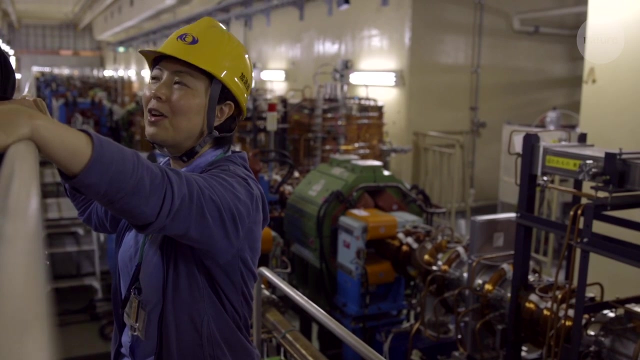 This is an accelerating cavity. Quad dipole, Six dipole, Two beam pipe. This one is four injected beam. injection beam, This one is a rotating beam. Wave guide, That pipe that is also wave guide. The steering magnet. 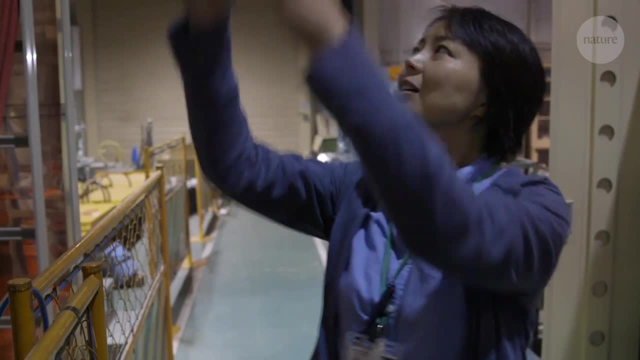 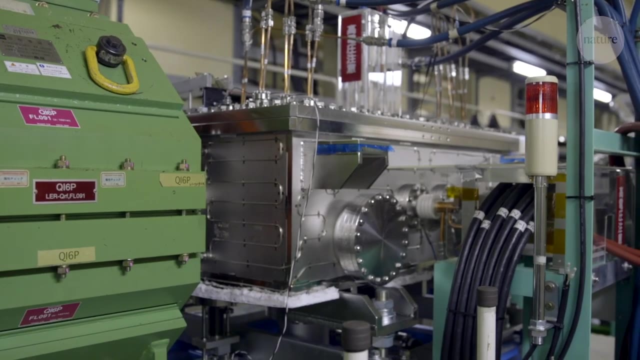 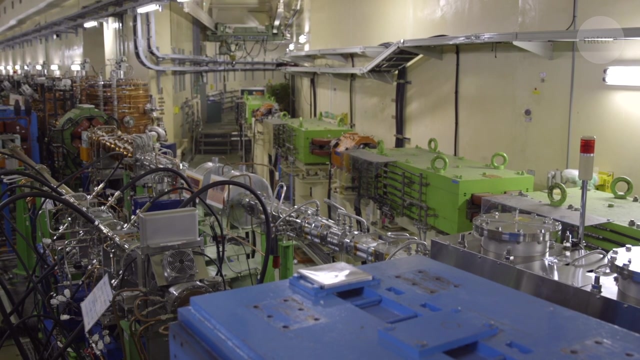 This is crystron And this is a cooling tower. We have four crystron in this building. And then we reach this point, The positron injection line. This is literally an antimatter injector, So you can see the injection line.